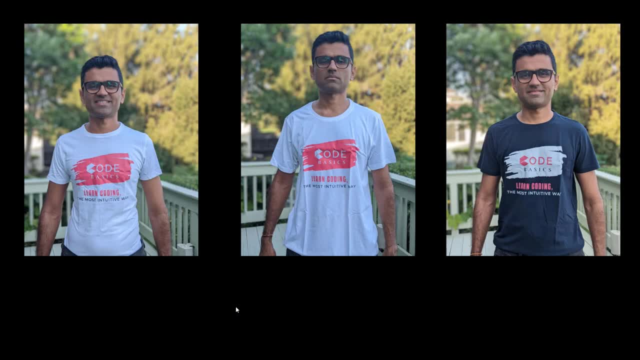 I'm going to explain bias and variance using a very simple language, and you are already wondering what's the meaning behind showing all these three pictures. Well, look at the pictures carefully and try to find out what I want to show you here. The first picture, of course, shows a t-shirt that I'm wearing, which is which: 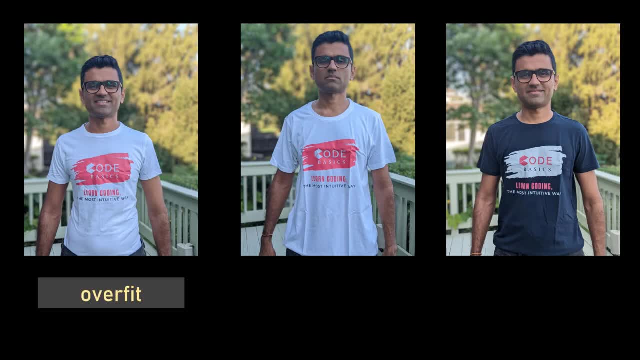 is too much fit. basically it's over fit. so if my body increases or decreases, you know, if I start eating junk it will not fit. The second one is under fit, which is too loose. basically you look at my sad face here. clearly it indicates what's. 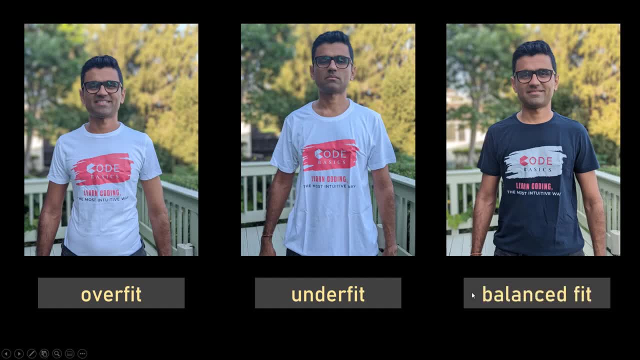 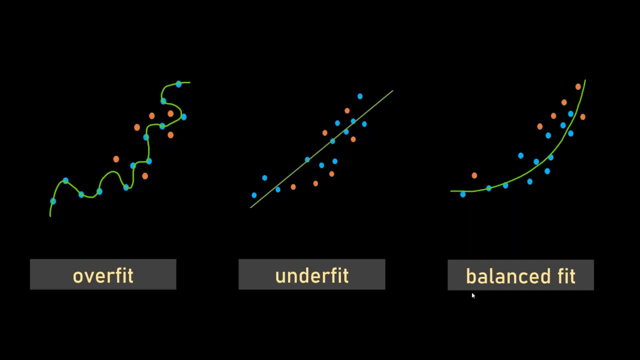 the issue here. The third t-shirt, however, is a perfect fit, where even I grow in size a little bit, or if I, you know, thin up a little bit, it's gonna be okay. Same concepts apply in machine learning world, where your model can be an over fit, under fit or balance fit, and we are 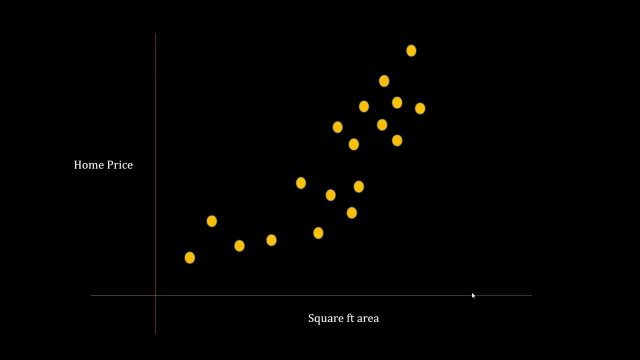 going to look at these scenarios using a simple housing price prediction example, where we are using one feature, which is the square foot area of a home, and based on this feature we are trying to build a machine learning model that can predict the home price. Here I have a scatter plot of all my training data set. 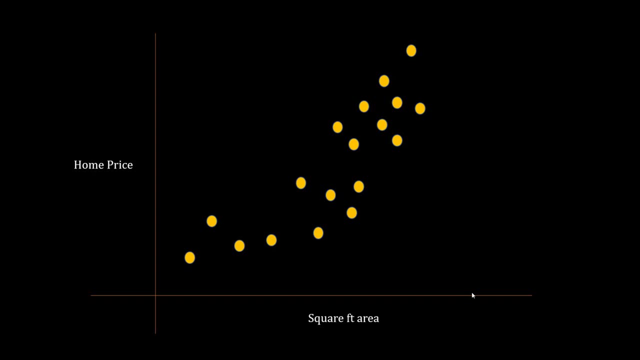 basically my data set super for the supervised learning. and in this scatter plot, when we train our model, what we do is we split this data set into training and taste samples. Let's say, all these blue dots are my training samples, the orange dots are my taste samples, and we can train a model. 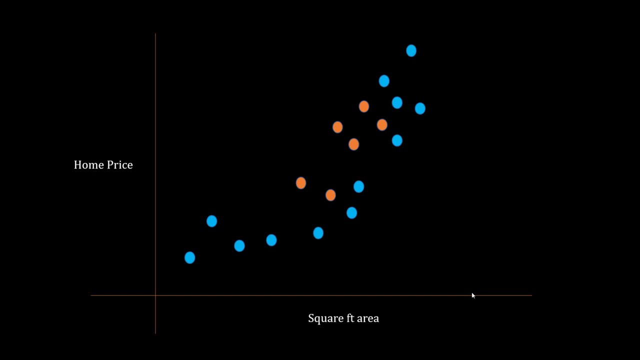 that fits to these blue dots. and let's say, our model is such that our training methodology is such that we train data set using a data set super for specialized learning model. we end up in an overfit model and overfit model tries to fit exactly to the training samples. 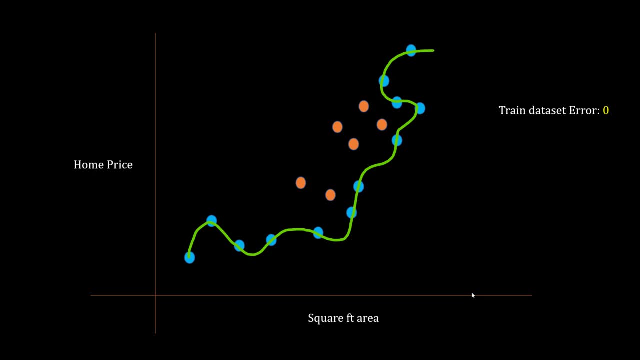 where your training error becomes close to zero. but the problem here is the taste error can become high because once you have this model train, which is this green line- now, let's say you want to figure out an error for this particular orange taste data point, the predicted value will be: 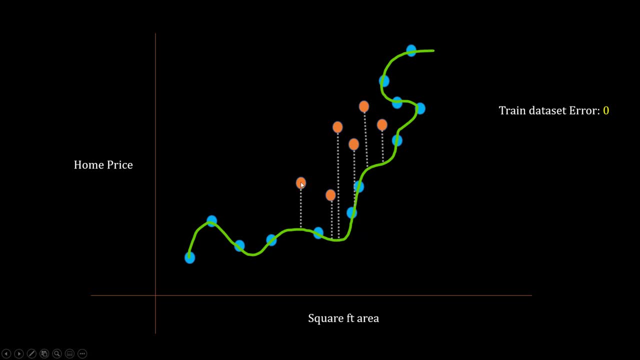 somewhere here and the error will be this gray dotted line and you can measure the error for all your test data set and average it out. let's say you get this error as 100. i'm just making this up. let's say this error is 100.. now remember one thing: when you have a data set and when you 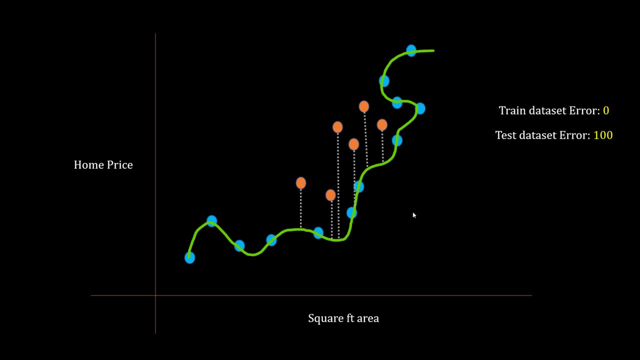 pick your training samples. you pick it up at random. you have trained test split, let's say 80, 20 percent. you pick your training samples at random. there's a different data scientist. they might be choosing different set of training sample- let's say this- and their model might look different. here they're using the same model. 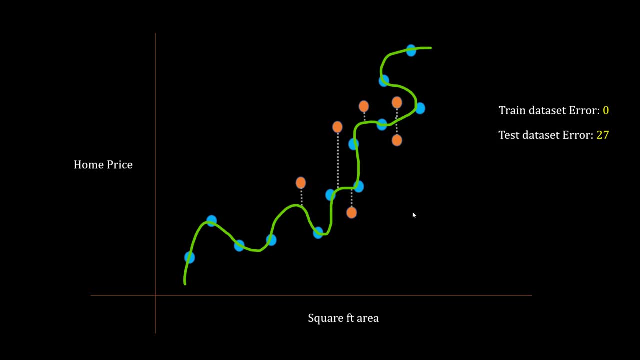 same methodology. so your training data set error is still zero, because you both are trying to over overfit the model. but the problem that happened here is your taste. data set error is, let's say, 27.. you can compare these two images and you can easily see. 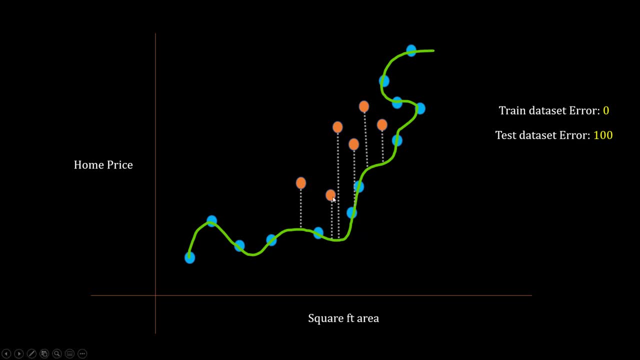 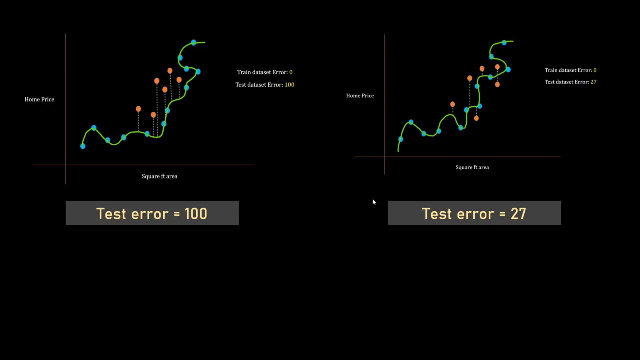 that the taste data set error here is much higher than the second scenario. you see, all this, you just sum up all these gray dotted lines here and some of the gray dotted lines here. this error is much less than the previous error. so if you compare these two scenarios side by side, in one case your 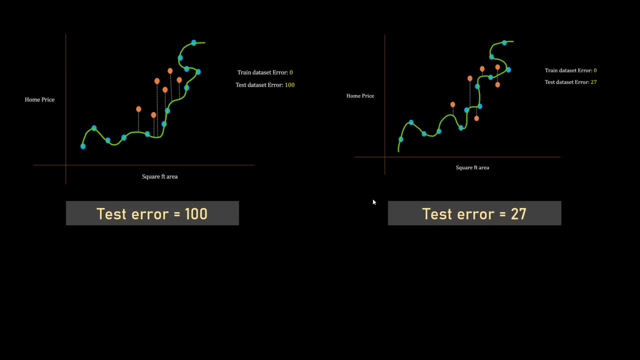 test error is 100. second case: taste error is 27, which means the taste error varies greatly based on your selection of training data point. and this is called high variance, because there is a high variability in the taste error based on what kind of training samples you are selecting. 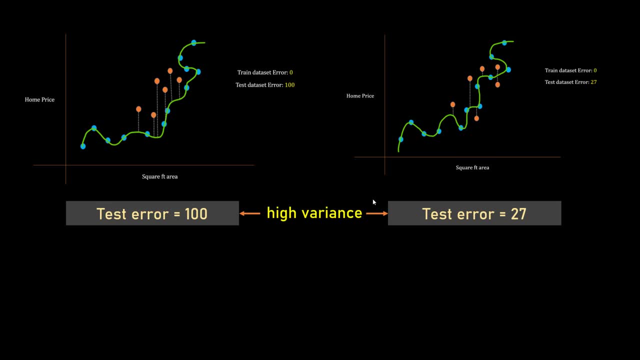 now you are selecting training samples at random, so your taste error varies randomly, which is not good. and this is the common issue with overfit model: they tend to have high variance. so high variance- again just to summarize- is high variance happens when your taste error varies by great deal. 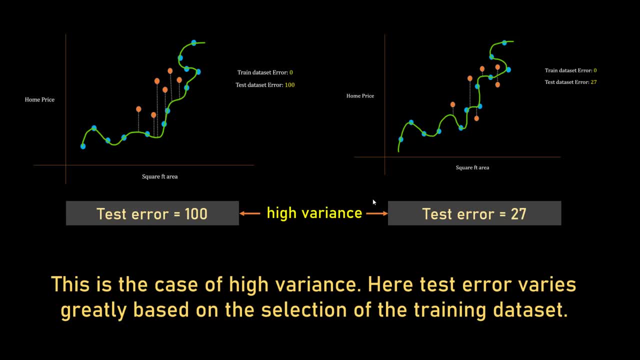 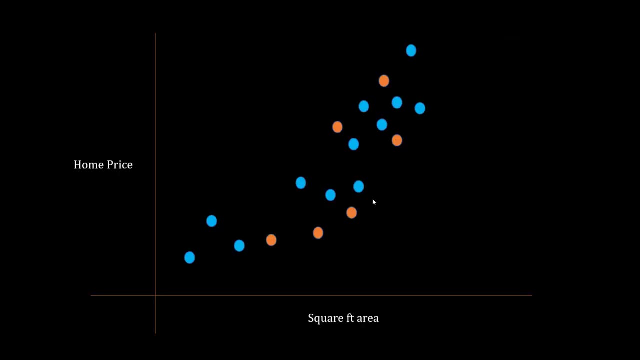 based on your selection of training data points. so just to remember, when you're talking about variance- high variance- you are always talking about taste error. let's look at another scenario where i have same data set, i have split into train and test samples and this time, instead of having a 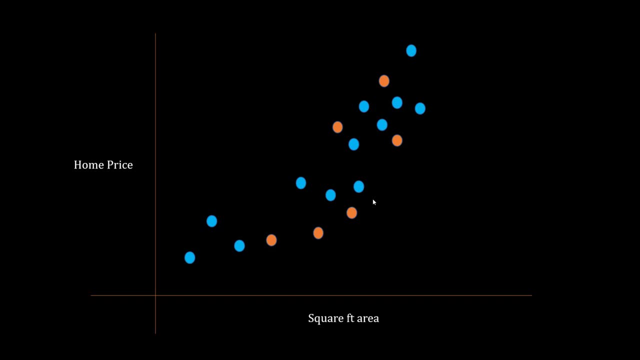 complex model that over fits my training samples. i'm trying to come up with a very simple model, let's say linear equation, which which is under fitting your training sample, because linear equation is straight equation. it cannot truly capture the pattern in your training samples. okay, the straight line cannot pass through all the blue dots. so it's a simple model where your 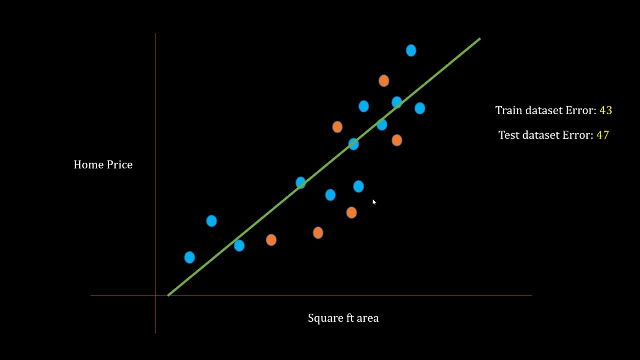 training error is actually high. in previous case, the complex model was complex. your training error was zero. here it is less than 43 and your test data set error is around 47.. again 43, 47- these numbers i just made up to explain you this concept. when you select a different set of training, 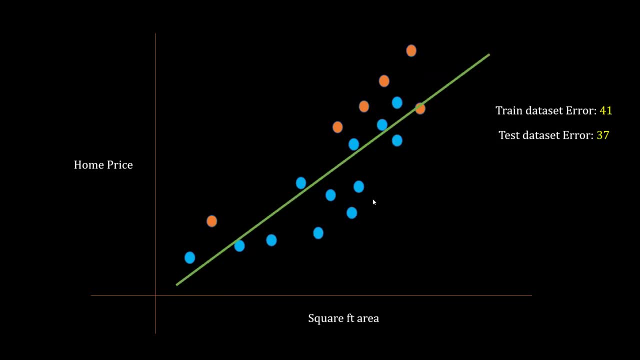 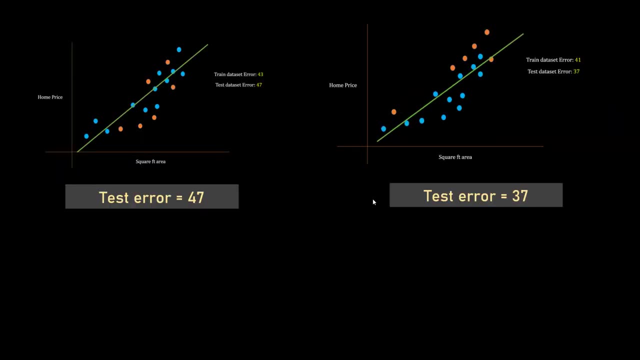 data points. see, in both the cases the line will be different, but your training and test data set error is still kind of similar. you know, in the first case it was 47, second case it was 37. so this is called low variance because based on what data point you select as your training samples. 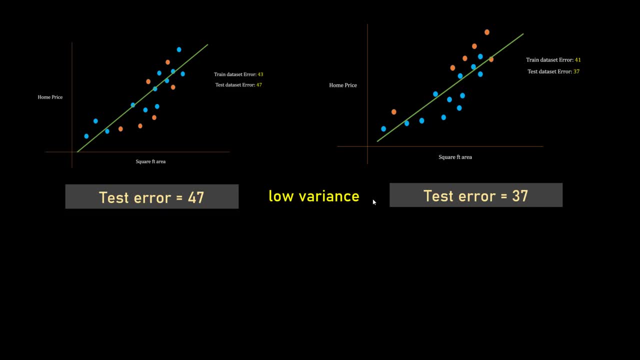 your taste error doesn't vary that much: 47, 37, they're still similar. it's not like 100 and 21, you know. so your taste error doesn't vary too much, hence low variance. but if you look at your train error, in the previous case your train error was zero. here you have some big train error. 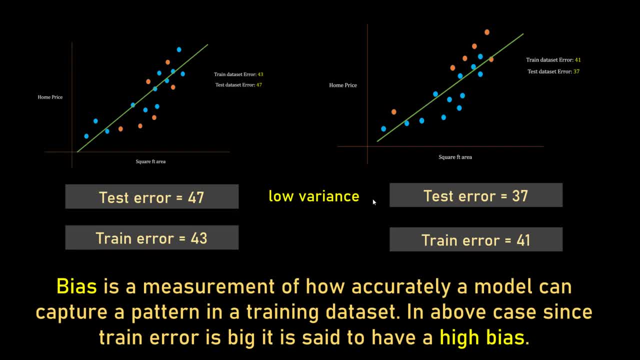 and that is called high bias. high bias is a measurement of how accurately a model can capture a pattern in a training data set. so when you're thinking about bias, you're always thinking about train error. when you're thinking about variance, you're always thinking about test error. bias is basically your model's ability to 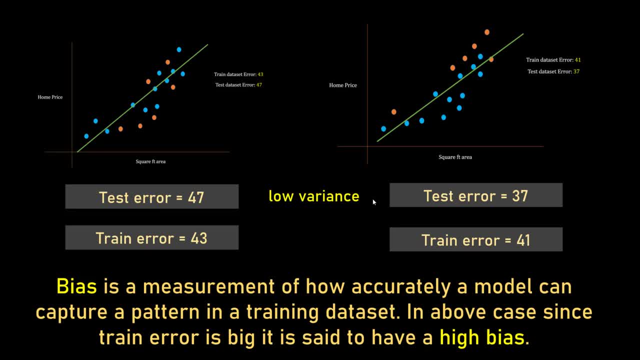 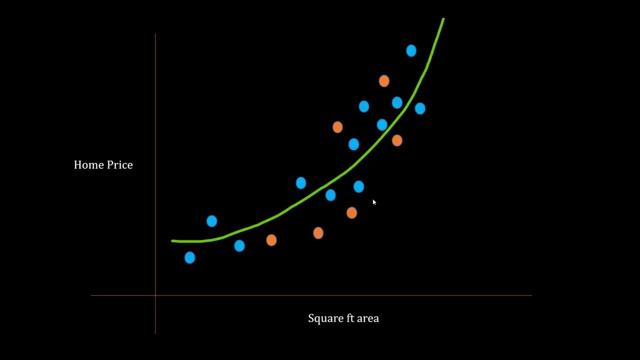 capture the pattern in your training data set in an accurate way. in the previous case where we had over fit the model, the bias was low because the train error was close to zero. so if, if the higher the train error, higher the bias. okay, now let's look at the idle scenario where you come up with 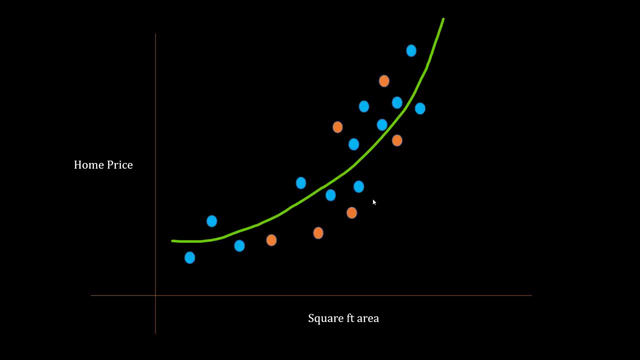 a model that kind of accurately describes the pattern that is available in your training data set. here your training error and taste error- both are low, even if you select different set of training data points- see the training data points here are different- but still your model selection is such that 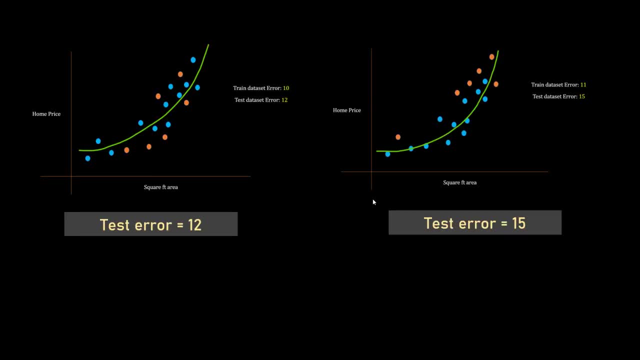 your train and test error. both are kind of low and in this case it's called low variance, low bias model, because your test error doesn't vary too much based on what training samples you have selected. also, your train error in general is low, so that's why it's called low bias. 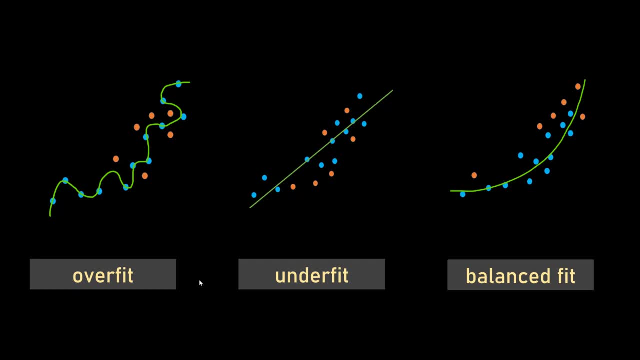 so we already covered these concepts, like whenever you have an overfit model, it's likely that you will get high variance. when you have underfit model, it is likely that you will get high bias. and when you have balanced fit, you will get low variance, low bias and, as a 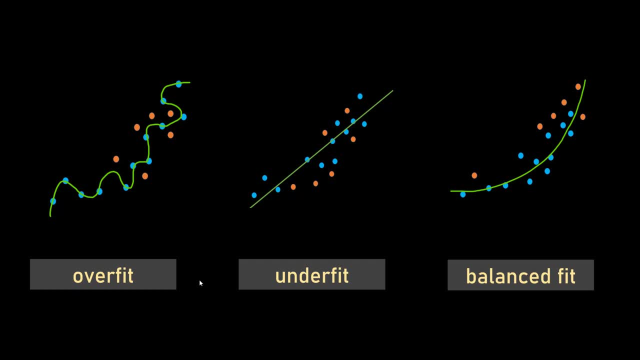 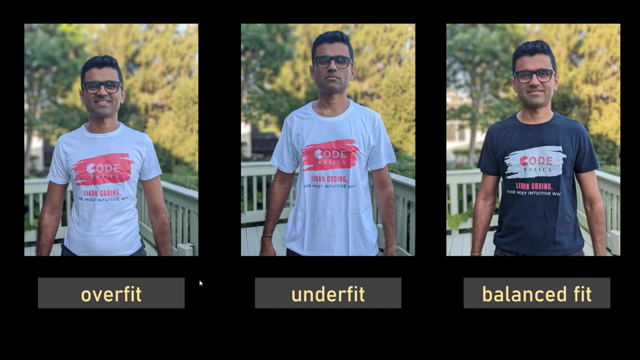 data scientist. you want to come up with a, with a model that has a balanced fit. you know, just like a t-shirt, you want to go to a store and buy a t-shirt. you will always buy a balanced fit t-shirt. now there is a bull's eye diagram where 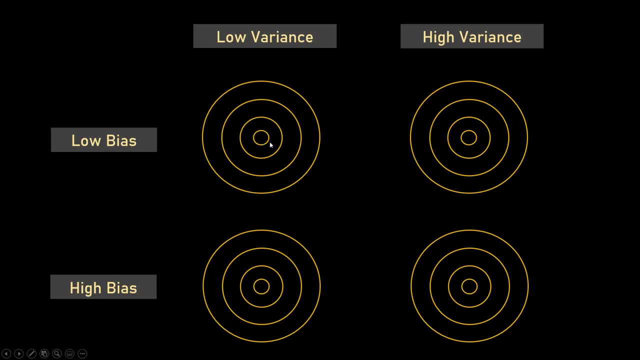 the central circle represents the truth. this is your truth. samples, okay, and when your predicted values. so these white diamonds are, let's say, your predicted values when they are near to the inner circle, which is a truth. it is called low bias. bias is all about how close you are to the truth. so if you are closer to the